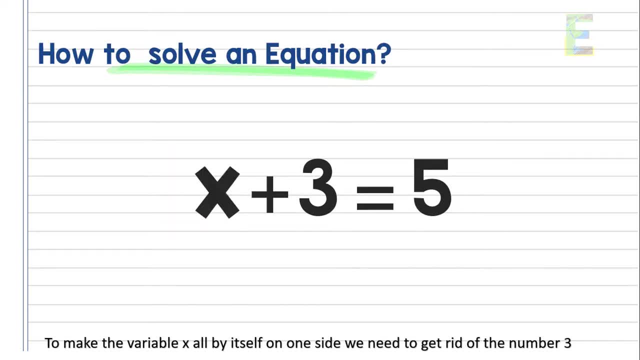 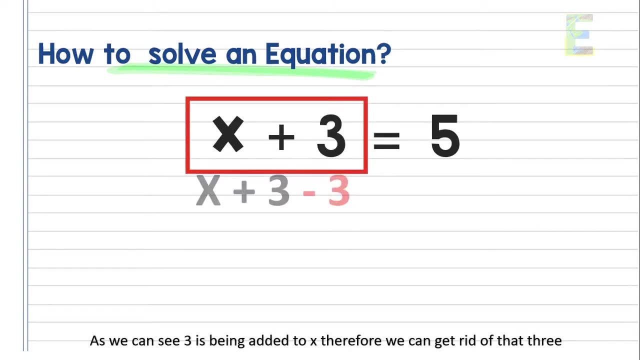 To make the variable x all by itself on one side we need to get rid of the number 3.. As we can see, 3 is being added to x. Therefore we can get rid of that 3 by subtracting 3 on that side. 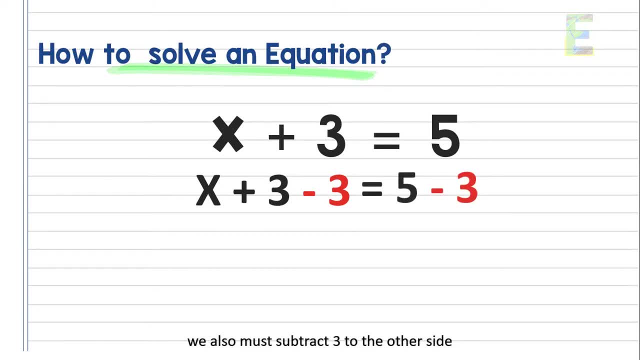 And to keep our equation balance we also must subtract 3 on the other side. So the x is now all by itself on the other side of the equal sign, because positive 3 minus 3 cancels out. Therefore our equation will become: x equals 5 minus 3.. 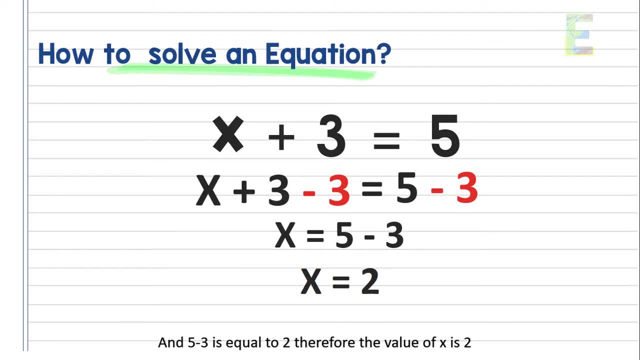 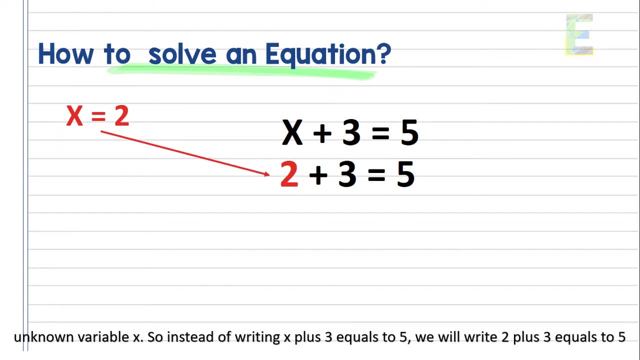 And 5 minus 3 is equal to 2.. Therefore, the value of x is 2.. And to check whether we got the correct value of x, we just need to substitute the value to the unknown variable x By the writing x plus 3 equals to 5,. we will write: 2 plus 3 equals to 5.. 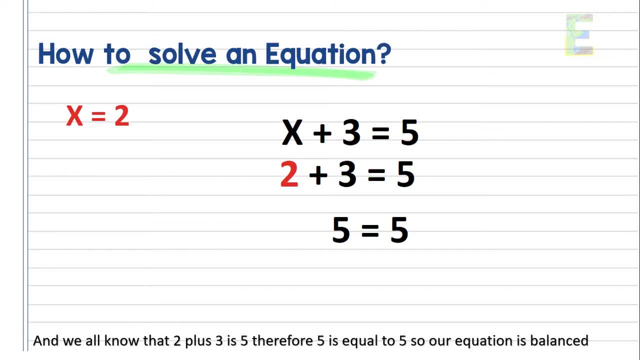 And we all know that 2 plus 3 is 5.. Therefore, 5 is equal to 5.. So our equation is balanced And we all know that we got the right value of the variable x. Let's have more examples to further understand it. 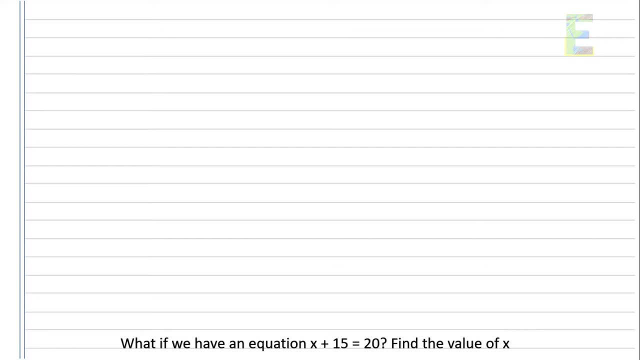 What if we have an equation: x plus 15 equals 20? Find the value of x. So, as what I mentioned earlier, we need to put the variable all by itself on one side of the equal sign And then all the known variable to the other side. 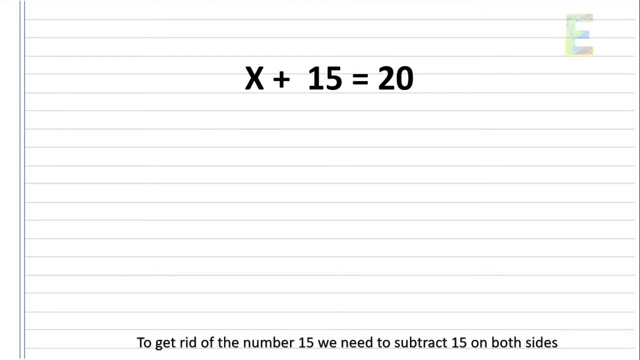 To get rid of the number 15, we need to subtract 15 on both sides, So the equation will become x plus 15 minus 15 equals to 50 minus 15.. And we all know that positive 15 minus 15 cancels out. 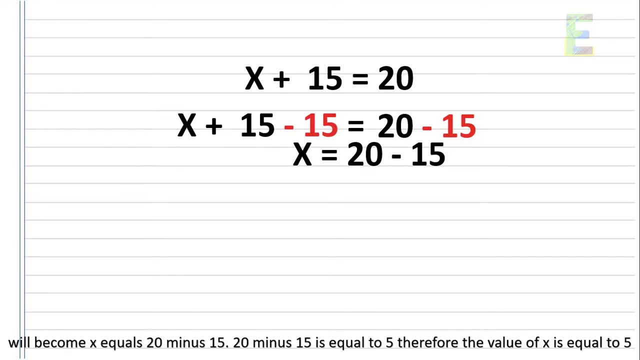 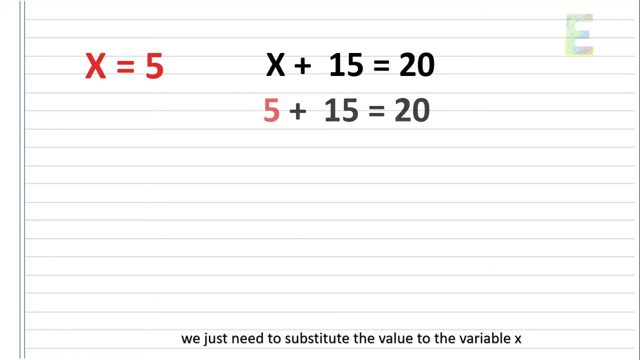 Therefore, our equation will be like this: Therefore, our equation will become: x equals 20 minus 15.. 20 minus 15 is equal to 5.. Therefore, the value of x is equal to 5.. To check whether we got the correct value of x, we just need to substitute the value of the variable x. 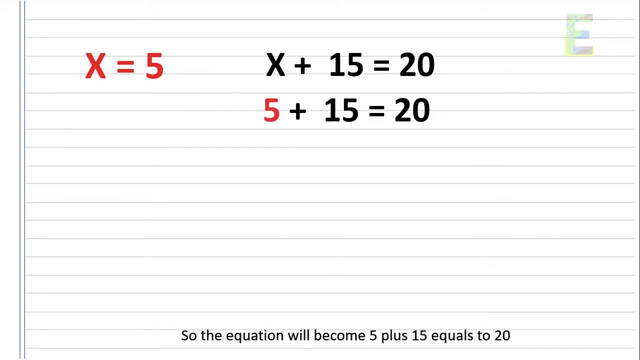 So the equation will become: 5 plus 15 equals 20.. And we all know that 5 plus 15 is equal to 20.. Therefore, 20 equals 20.. So our equation is balanced And we got the correct value of x. 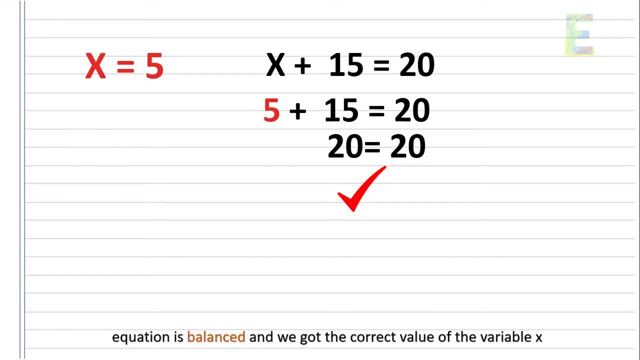 So now we have the correct value of the variable x. Okay, for another example, If we have an equation: x minus 9 equals 2. Find the value of x. Again, we need to put the unknown variable all by itself on one side. 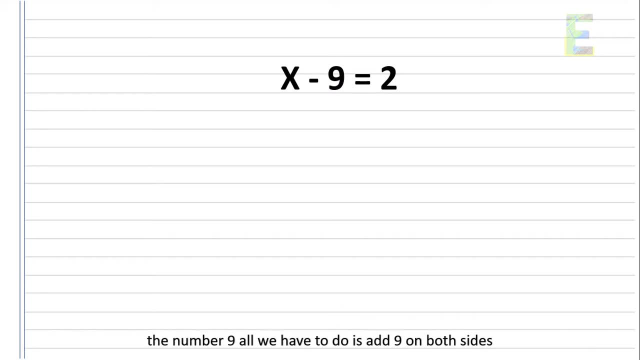 So, in order to get rid of the number 9, all we have to do is add 9 on both sides. Therefore, the equation will become: x minus 9 plus 9 equals to 2 plus 9.. positive 9 minus 9 cancels out, because 9 minus 9 is 0. therefore the equation will: 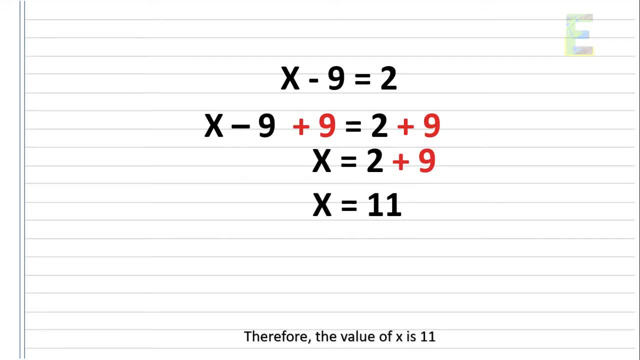 become X equals 2 plus 9. therefore the value of X is 11. and then to check whether we got the correct answer, we just need to substitute the value to the equation. so the equation will become 11 minus 9 equals 2. so since the equation 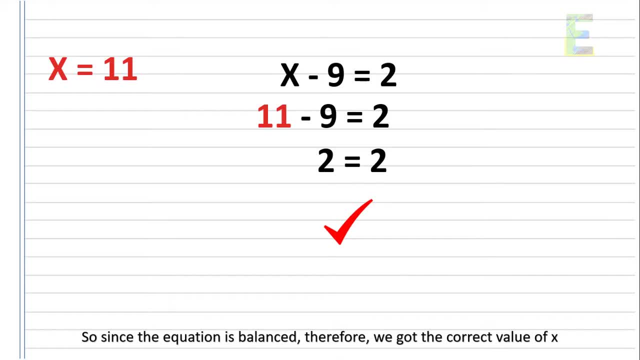 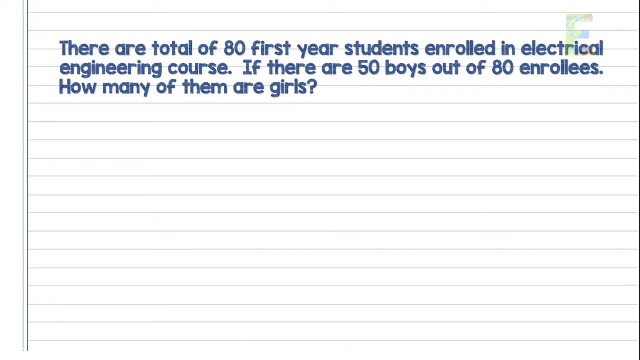 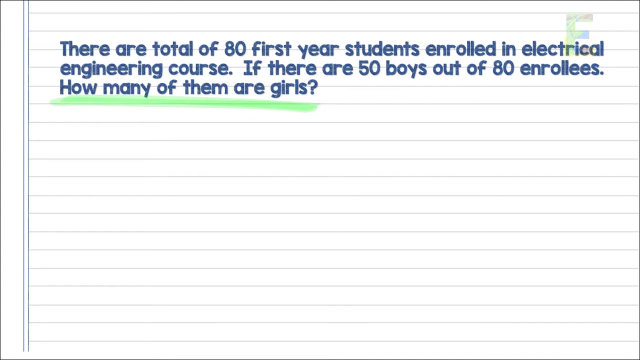 is balanced. therefore, we got the correct value of X. now let's have some word problems. there are total of 81st year students enrolled in electrical engineering course. if there are 50 boys out of 80 enrollees, how many of them are girls? I will give you 30 seconds to solve this problem or you can pause the. 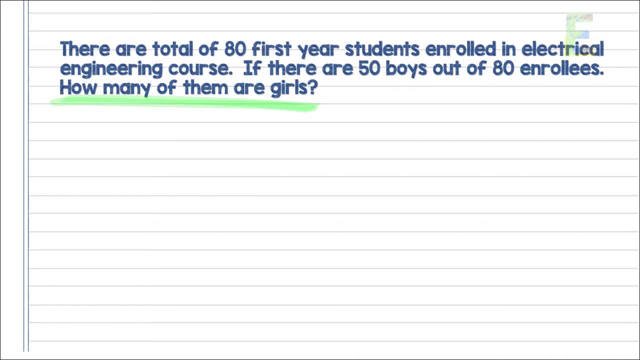 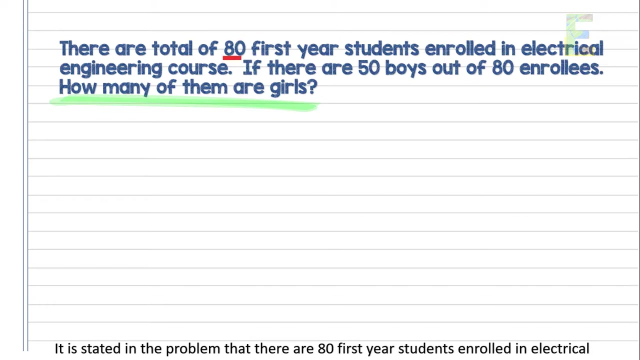 video. if you need more time, so time I will give you 30 seconds to solve this problem, or you can pause the video if you need more time, so time starts now. it is stated in the problem that there are 81st year students enrolled in electrical engineering course and 50 of them are boys, and the problem is asking: 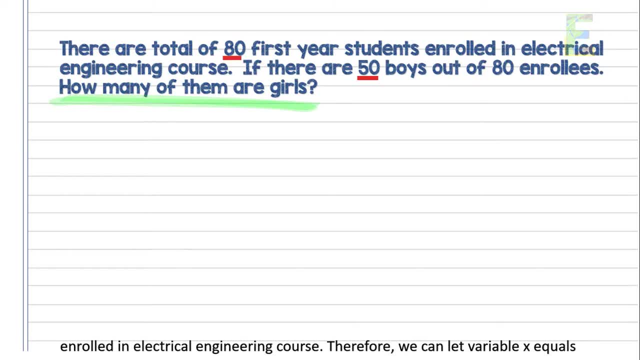 for the number of girls enrolled in electrical engineering. therefore, we can let variable X equals the number of girls enrolled in electrical course, and since the total number of enrollees is 80, therefore we can conclude that the total number of boys plus total number of girls is equal to 80 students. so this will be our equation to get the value of.